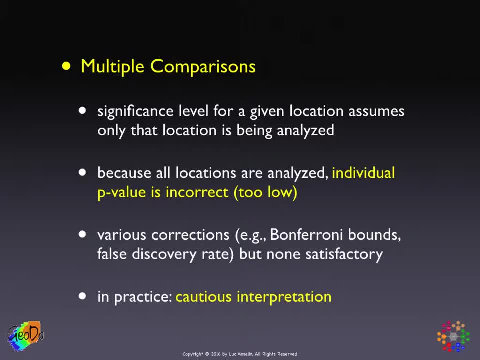 So if you do a local analysis on 3,000-some US counties, you would have to divide your target p-value by 3,000.. To have the actual value that you would use for each individual comparison And the question. 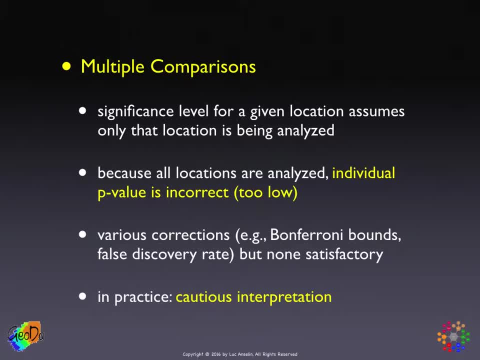 then arises: should it really be 3,000, or should it be a smaller value, maybe the number of neighbors or the average number of neighbors? And so none of this is actually very good. My recommendation and my rule of thumb in practice is just to be cautious, and by all. 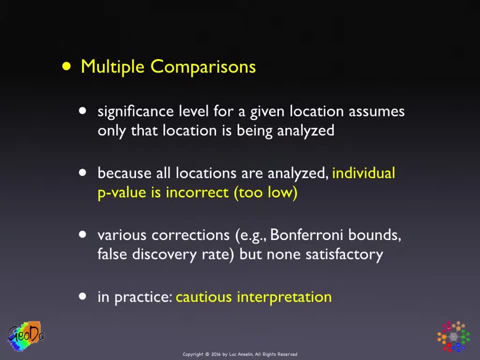 means: don't get too excited when you get a p-value. Okay If you get a p-value of 0.05.. On the other hand, as we've seen when we compare the different maps of the clusters and also the core of the cluster, together with the neighbors, at the end of the day they all 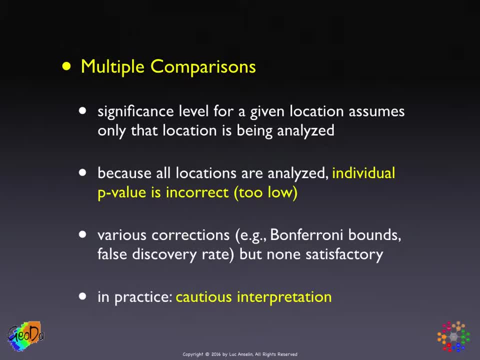 seem to point in the same direction. So even if you take a much more stringent p-value, such as maybe p.001,, if you add the neighbors to the cluster's cores, then you end up with something that's very similar to the indication given at a higher p-value. So the rule is: 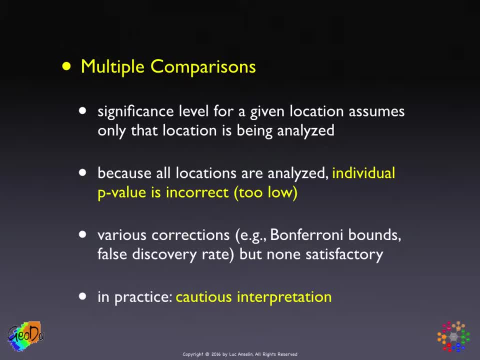 to be cautious is to do sensitivity analysis and is to be aware that these p-values, first of all, they're only pseudo p-values, so they're not really the real thing to begin with, but also they only give you an approximate sense of the significance. However, if you find 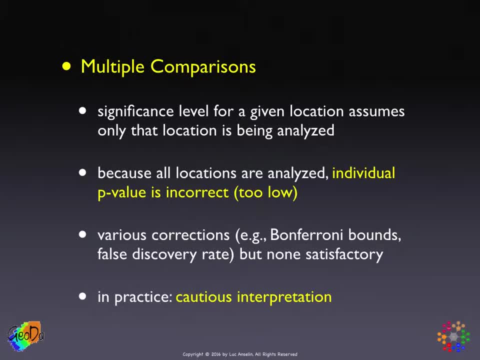 p-values that are 0.0001, then there can be a fair degree of confidence that you're onto something. Now, whether the degree of uncertainty as measured by the p-value is exactly what you have there, that almost surely is not the case. What it is exactly is also: 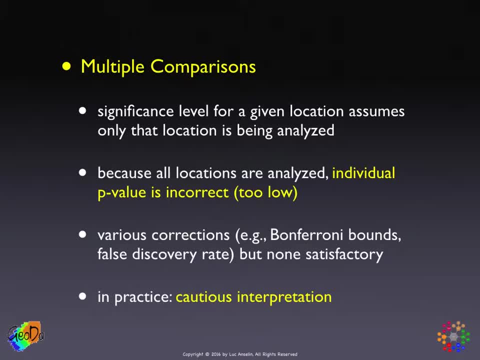 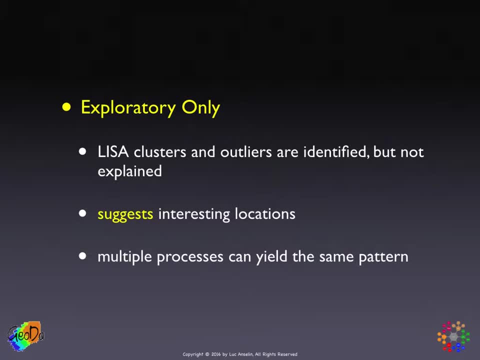 almost surely impossible to determine. So that's the first issue to keep in mind. The second issue is this, not to make too much of it again, this is just an exploratory technique. The clusters and the outliers are identified, but they don't actually explain. 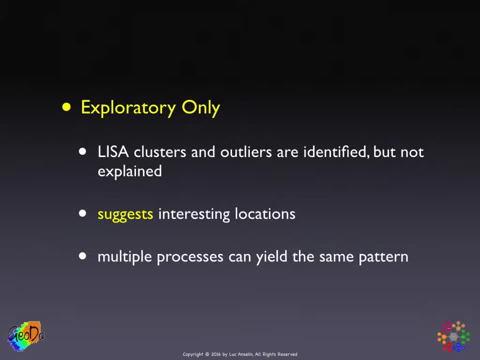 anything, And it's important to keep in mind what we discussed earlier, also for the global space-loader correlation measures, that the cluster detection is about pattern and not about the process. So just identifying the pattern you can't really say anything, or you can't say everything. 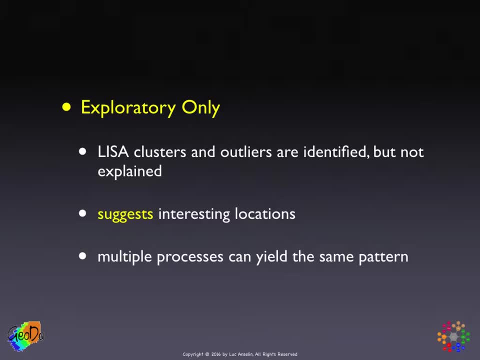 about the process, But we saw this in the context of pure against apparent contagion, where, in fact, just identifying clustering, or in our case just identifying a cluster, is insufficient to be able to draw the conclusion which of the two processes might have yielded this cluster. 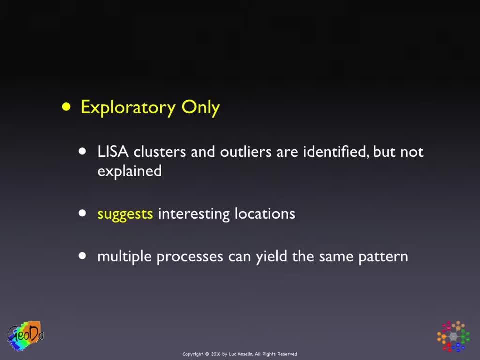 What it does do, though, is especially in an exploratory spirit, following the ideas of Tukey- is that it does suggest interesting locations. interesting locations which then should prompt you to look at other relationships and other variables that might potentially lead you to formal hypotheses. 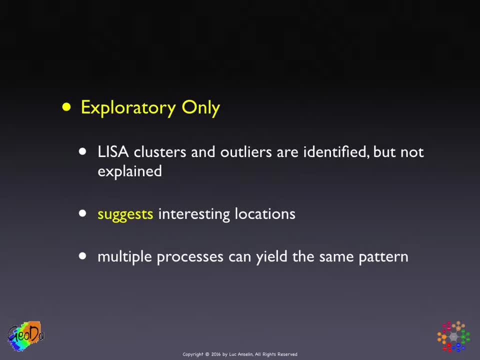 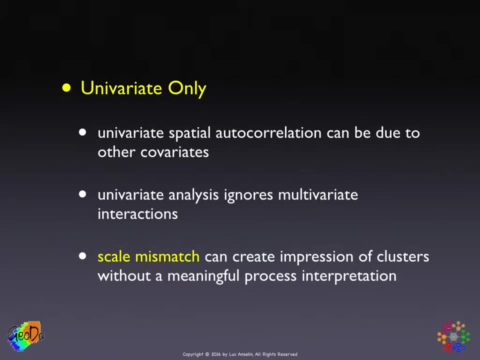 which can then be incorporated in actual modeling. So multiple comparisons, exploratory only, and then the final one. it's univariate, These clusters. they can be due to interaction effect with other covariance, and that is something that is always the case when you deal with a univariate statistic. 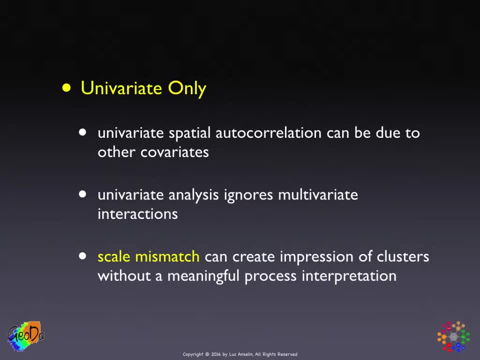 it ignores multivariate interactions. And there's another aspect to this: that scale mismatch can often create the impression of clusters that are actually they're there, but they're there because of data issues. There's no substantive, meaningful process interpretation, And an example that you often run into is with the analysis of housing markets. 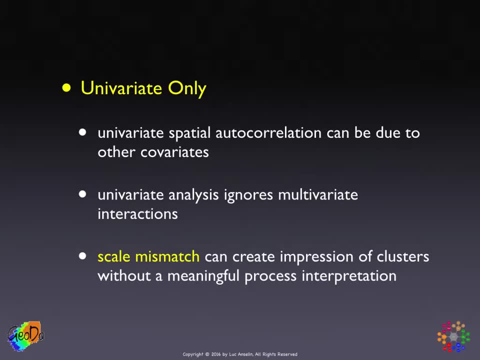 and I mention this often as a classic Example. if you look at housing developments in the US Southwest or in California, very often these developments are done in cohorts and thousands of houses are built at the same time, and they're all the same.